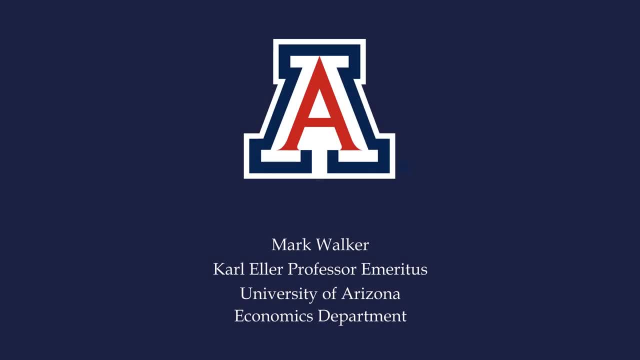 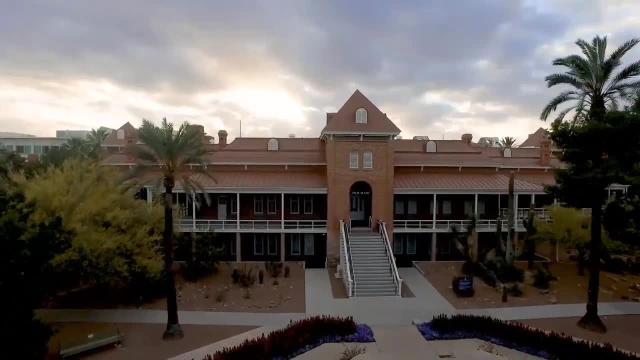 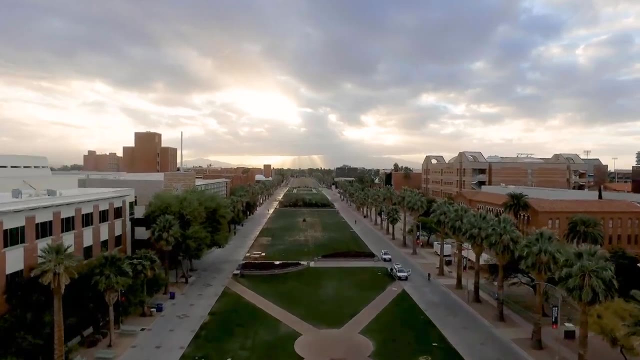 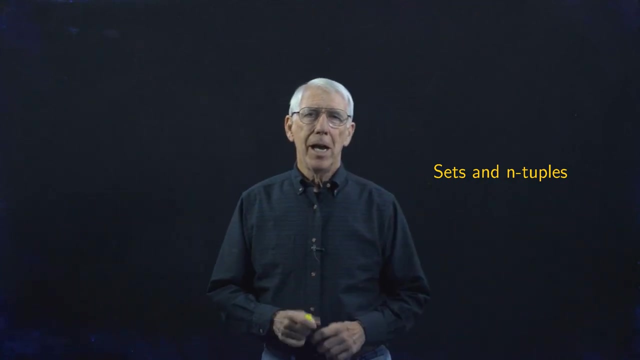 Hi everybody. I hope everybody's having a good day today so far. We are going to start out by spending a few minutes talking about sets and n-tuples. Now, in this first lecture, and probably for the first few lectures, a lot of what we do is probably going to be review for most of you. 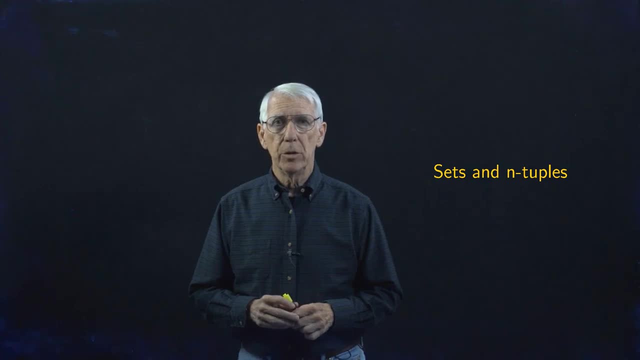 I say a lot, but probably not all of what we're going to do will be review, But it's still the case that, even though some of this is going to be familiar, it's still important for us to kind of do that review, to start out with things that are familiar and straightforward for us. 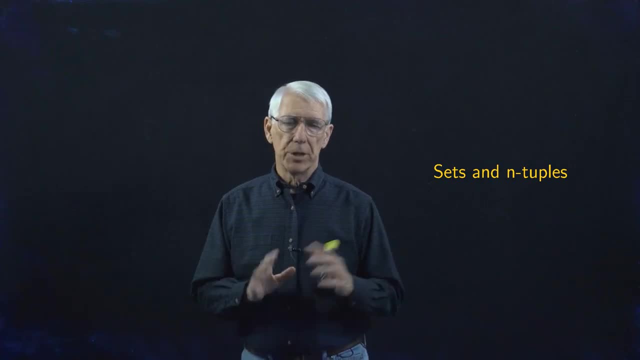 and also so that we all kind of get on the same page in terms of the concepts and the notation for those concepts that we're using. So let's start out by talking about the special sets and numbers that we use and the special notation for those sets. 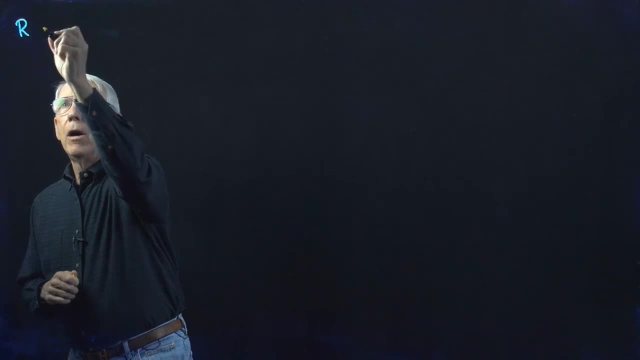 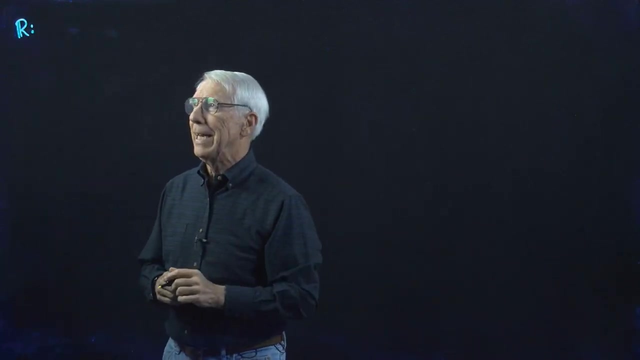 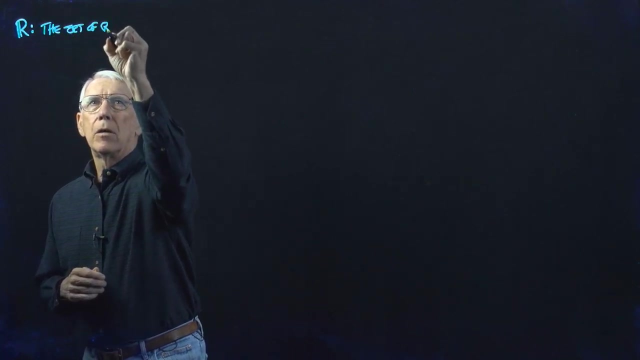 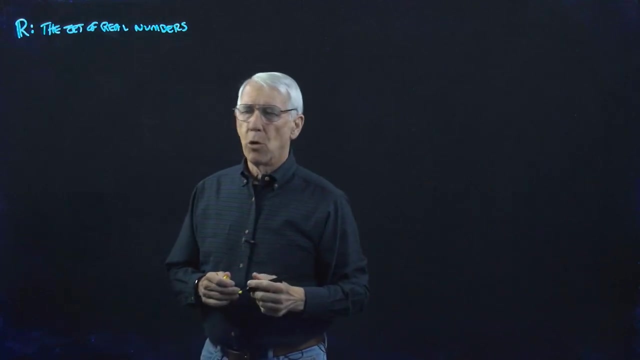 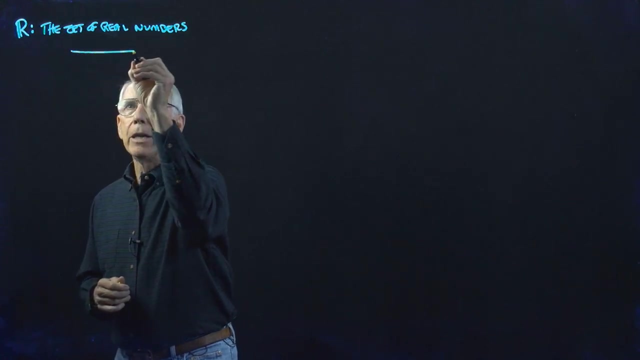 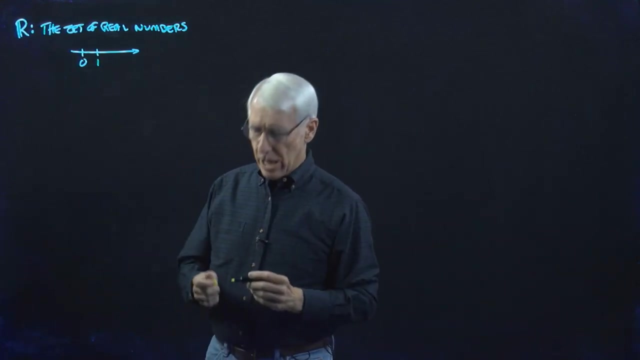 So let's start with R, the special kind of R, with the two lines on the left, And that's of course the set of real numbers. And we often, of course, represent the set of real numbers by geometrically, by a line, and we even refer to that line as the real line, often and kind of synonymously with R, the set of real numbers. 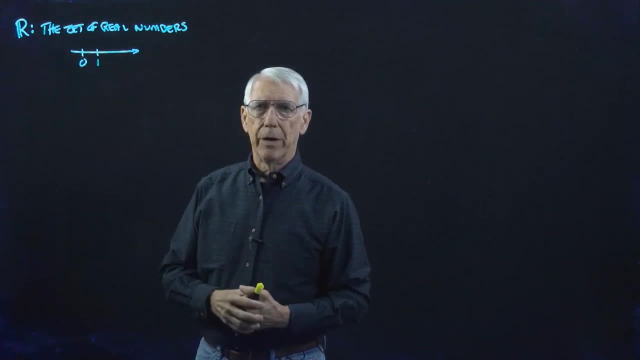 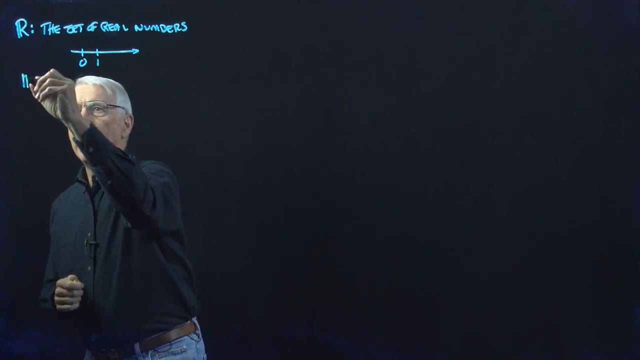 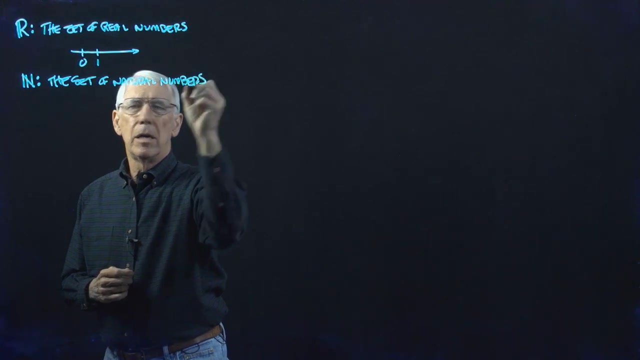 And we think of the elements of the real numbers as being the points on the line. And then we have the special symbol n, which is the set of natural numbers, And that is the set consisting of the counting numbers. natural numbers are the counting numbers. 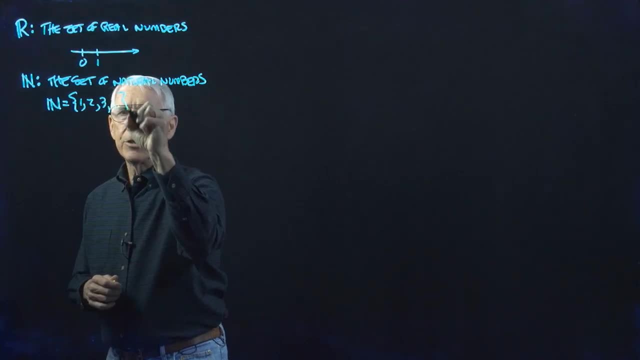 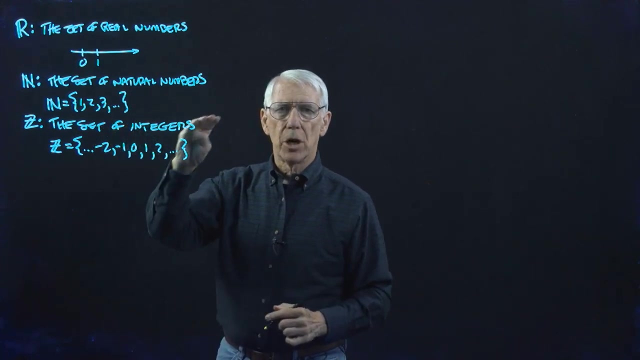 And so that's 1,, 2,, 3, and so on indefinitely. We have the set of integers, That is, the set of all the negative and positive integers and of course, zero. So the dot, dot, dot, ellipsis or dots here just indicates this goes on forever in the positive direction, this goes on forever in the positive direction and also goes on forever in the negative direction. 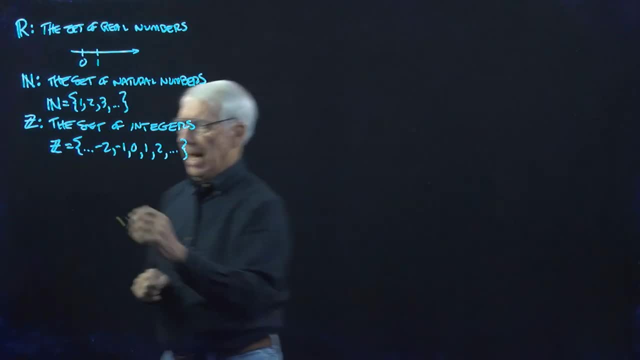 So that's 1,, 2,, 3, and so on indefinitely. And then we have the set of integers. That is the set of integers, That is the set of integers in the negative direction. And the remaining kind of special symbol that we use is this: Q. 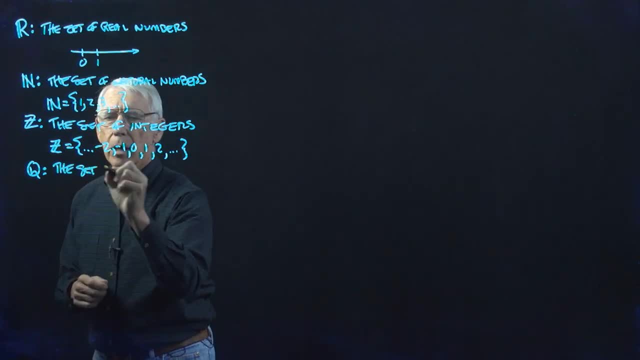 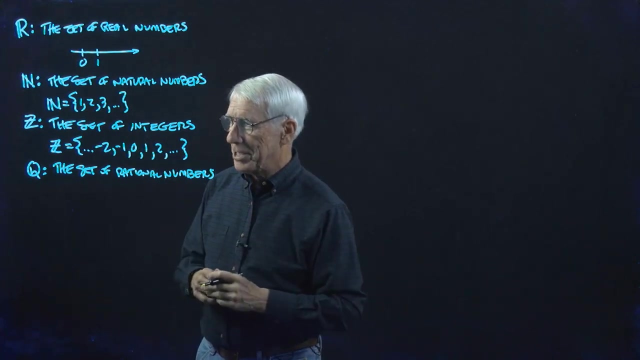 for the set of rational numbers. Why Q? I have no idea. I don't know why we use Q for the set of rational numbers. Maybe there's a reason. I've never, no one has ever. it's never come up really. 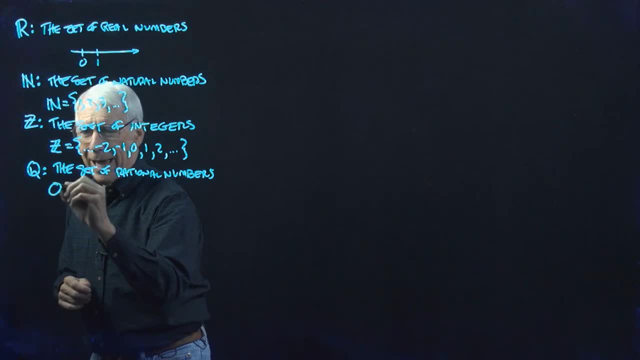 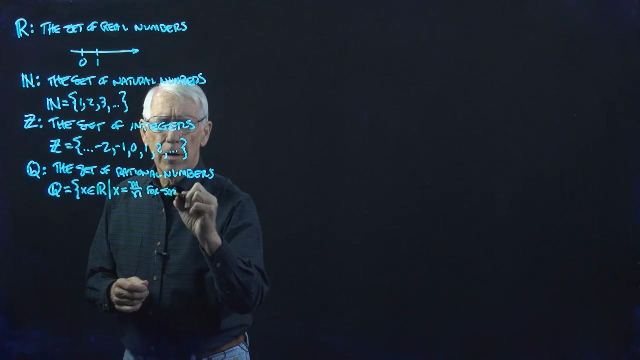 I guess before. So let's just point out that we can actually write down a definition of the set in this way: It's the set of all real numbers, such that x is a ratio of integers, So such that x equals m over n, for some. 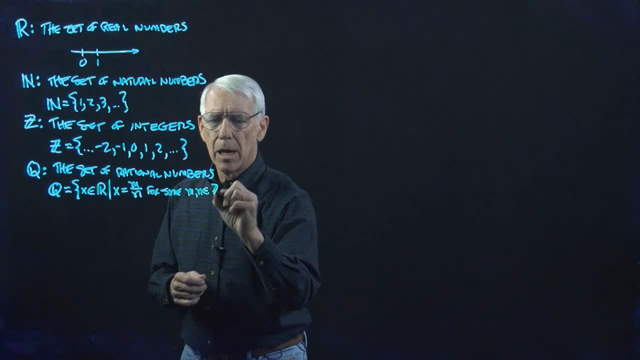 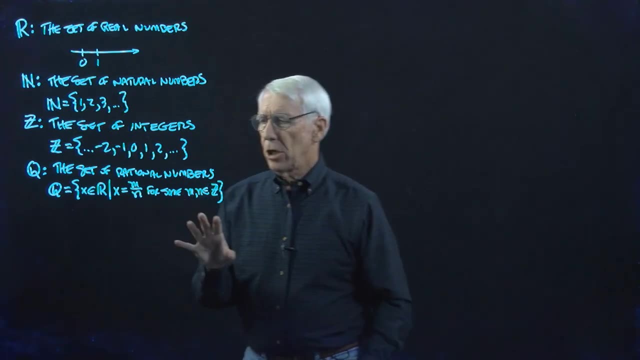 n, m and n in z. that is for some integers. Now this might look a little suspicious. You might be a little skeptical of this, because you could say: wait a minute. now one of the integers is zero, And if the 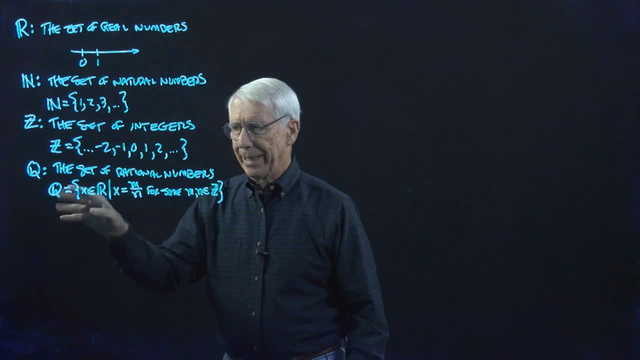 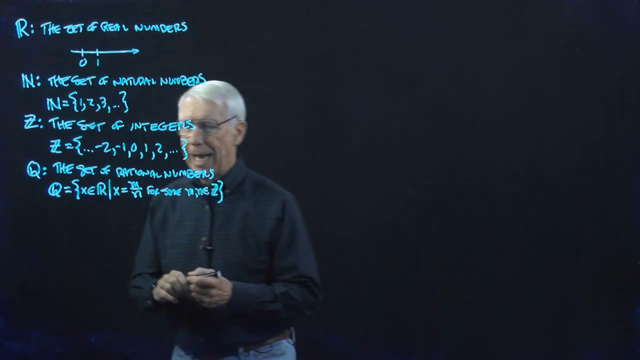 denominator is that integer. well then, we're not going to get a, we're not going to get a rational, we're not going to get any kind of number, because any, any integer divided by zero doesn't have any value. So you might say, oh, that doesn't look quite right, But that's actually not so. This is actually okay, And so let's see why that might be so. 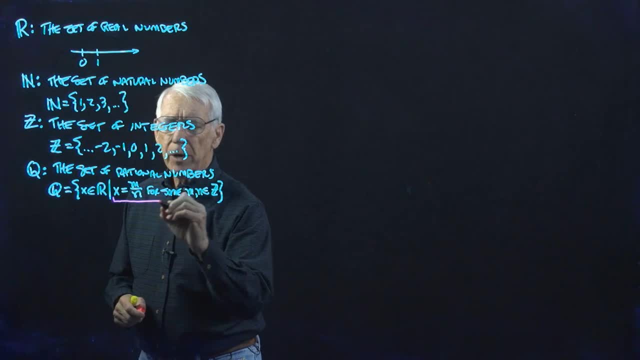 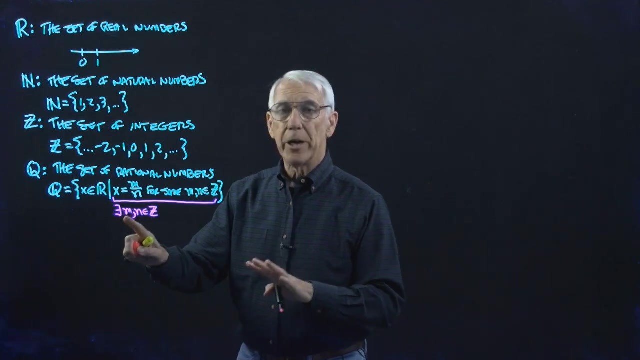 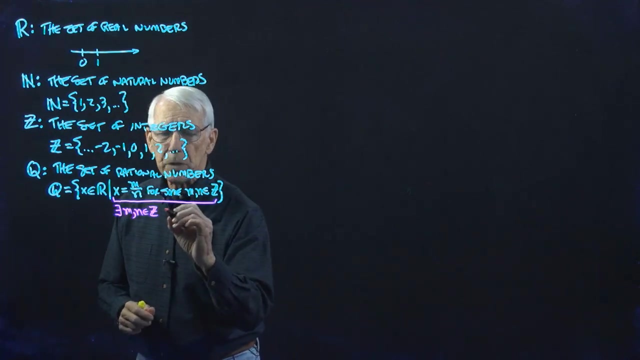 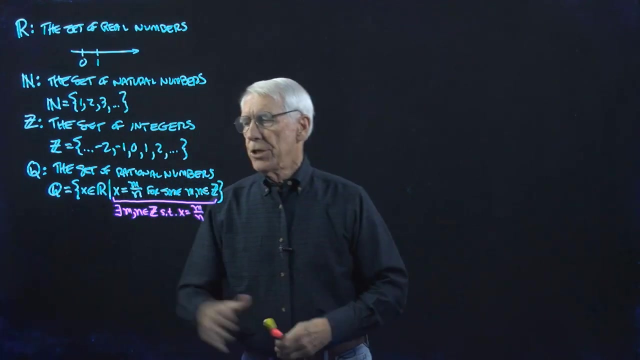 Note that I could rewrite the part over here, to the right of the vertical line, that delineates which x's we're talking about. I could rewrite this as follows: A backwards e, which we mean, which we read as there exists, there exists, I guess we'd say here there is exist, integers m and n, such that x equals m over n. So this is the. 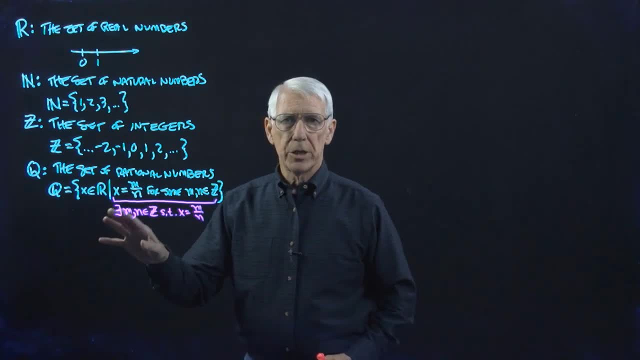 existential quantifier that we use all the time. We're going to talk about that in probably the next lecture, so I won't belabor anything about that here, but this simply is an alternative way to write what we have here. So it says it's the set of all real numbers, for which 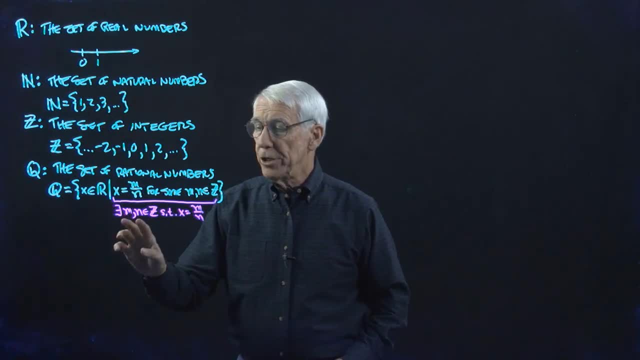 there are integers such that the real number is m over n. You can say, well, that really kind of looks the same and it actually is the same. but this perhaps makes it a little clearer that the zero is ruled out in what we've said here, because this says to set of all real numbers such that 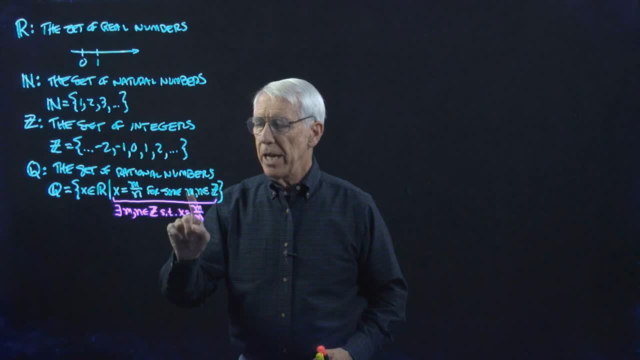 there exists an m and an n, such that the number is m over n, but of course, if there is no n, such that any real number would be equal to m over zero, there is no. if n is zero, then there is no m. that will go along with zero to give me. 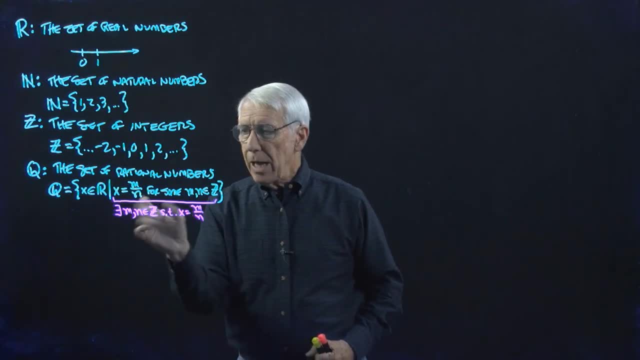 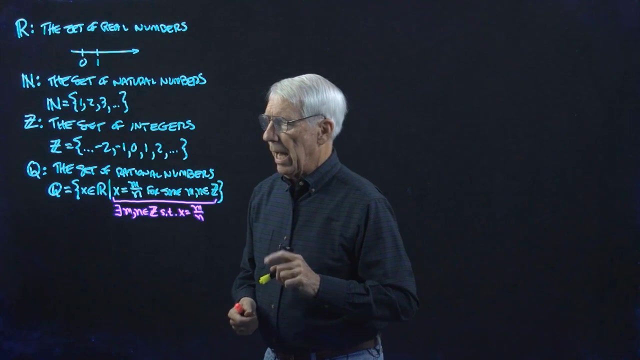 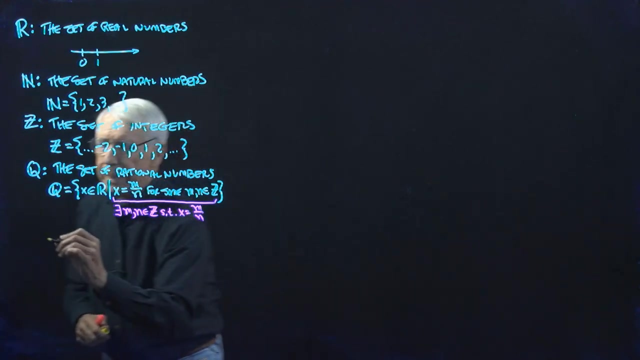 m over zero has a real number. So this is okay. It's just that the number zero, the integer zero, just can't show up in this ratio. Now there are there's a collection of additional special symbols for these sets that we should look at briefly, And 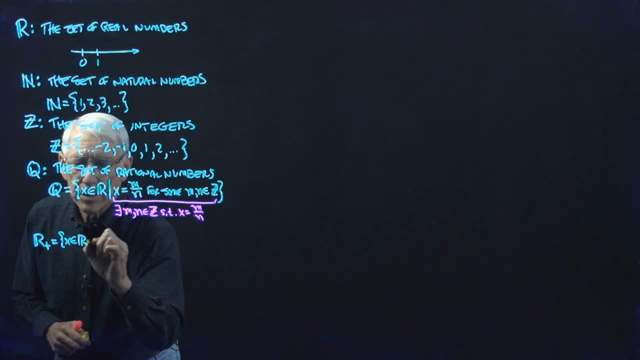 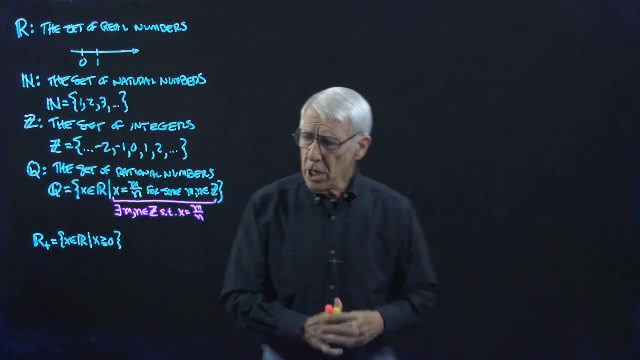 is the set of all real numbers, such that x is greater than or equal to zero. So it's just the non-negative real numbers And it's a little bit counterintuitive because you'd think with a plus down here then presumably this is the positive, strictly positive real. 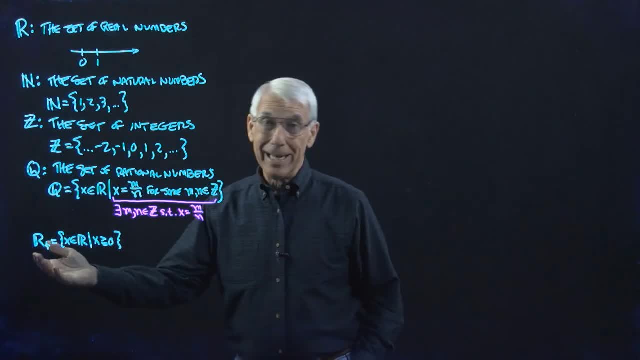 numbers And I think that would be the right intuition in some sense. But it just happens that the convention of the set of all real numbers is greater than or equal to zero. So the convention everybody uses is that r sub plus is the non-negative real numbers. 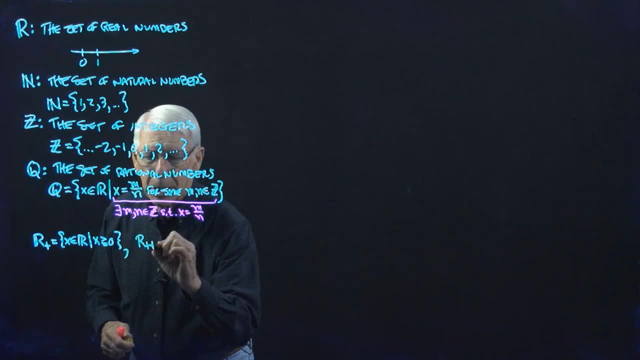 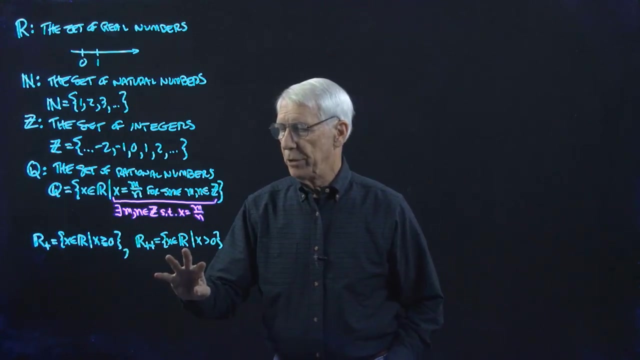 And we use r plus plus for the strictly positive real numbers. So this is so. this is the set: r plus plus the strictly positive real numbers. And of course we use the same notation occasionally for z plus and q plus to be the non-negative integers and the non-negative 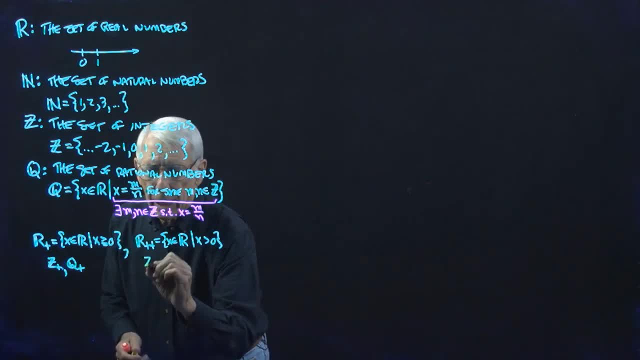 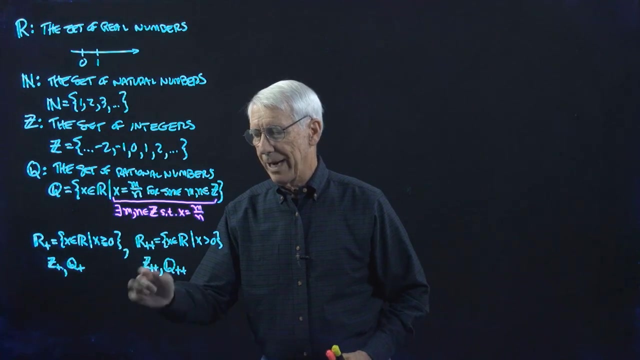 rational numbers And we sometimes use z plus plus and q plus plus for the strictly positive integers and the strictly positive rational numbers. And in fact I don't know if you've seen the graph of this. We probably don't know if we'll ever have to use this, because 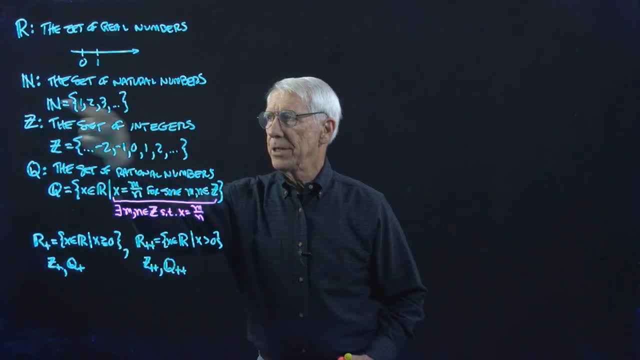 the strictly positive integers is the same thing as the set of natural numbers, So we would typically just use this. So these are just special symbols that we use for these particular special sets of numbers that we kind of use all the time. 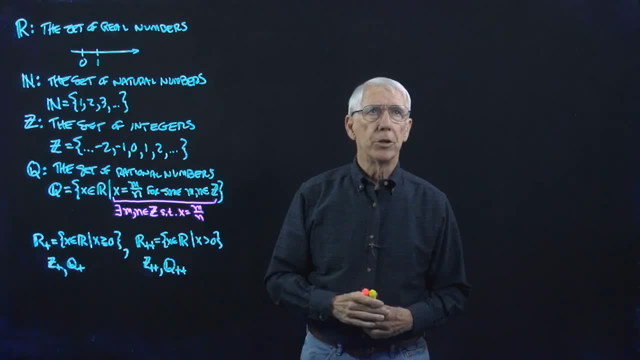 Now the next thing that I want to talk about here is that we can if we have a set x, so let's say, here we have x minus x. If we have x minus x, So here we have x minus x. So. 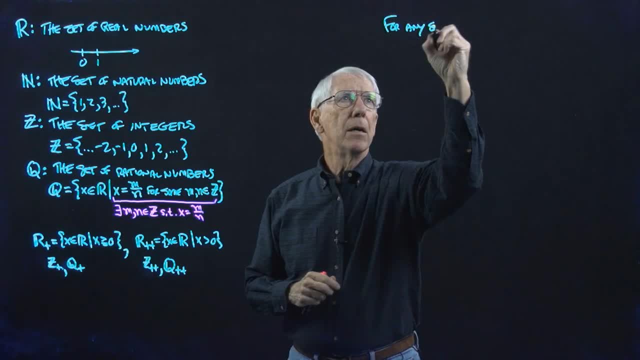 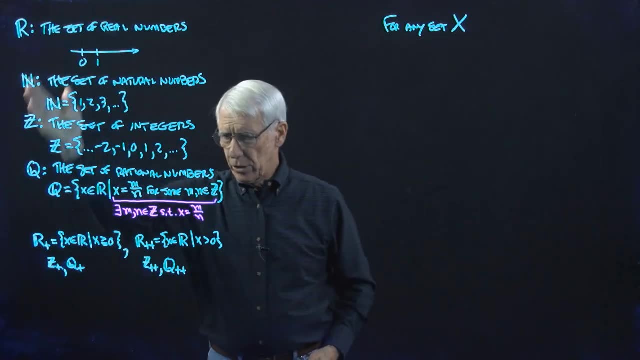 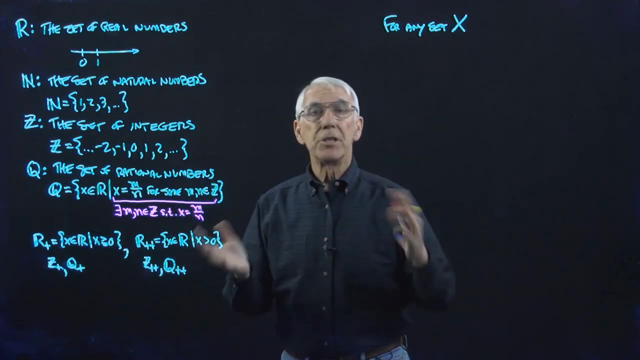 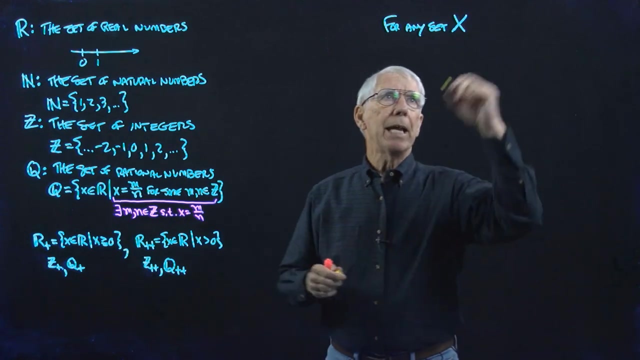 let's say that we have x minus x, And if we're, and here comes the initialz. and now, if we're here, for any set capital X, it could be R, it could be the rationals, it could be R plus plus, or it actually could be a set that doesn't consist of numbers. It could be a set of people, a set of colors, as we're going to see in a little while. For any set, X. 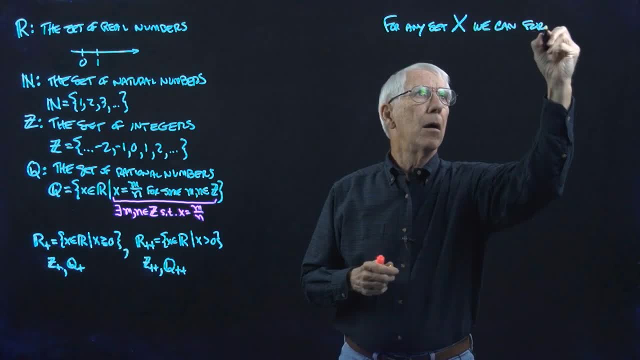 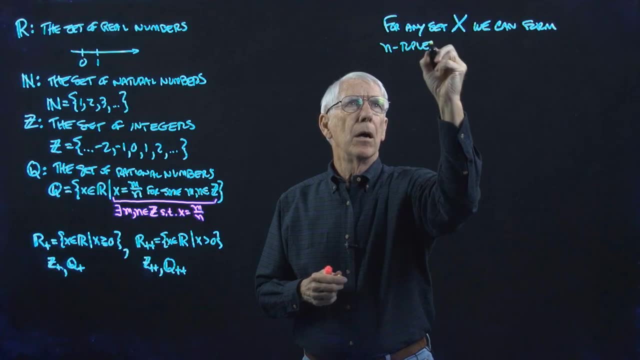 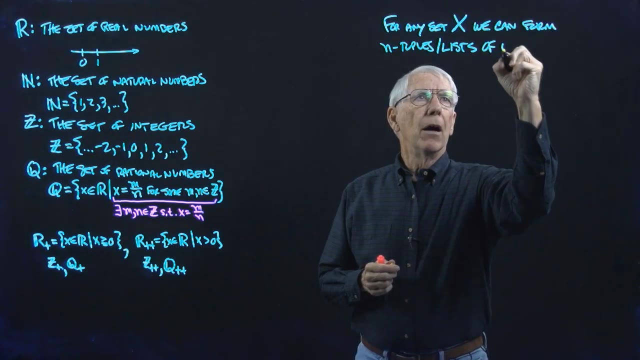 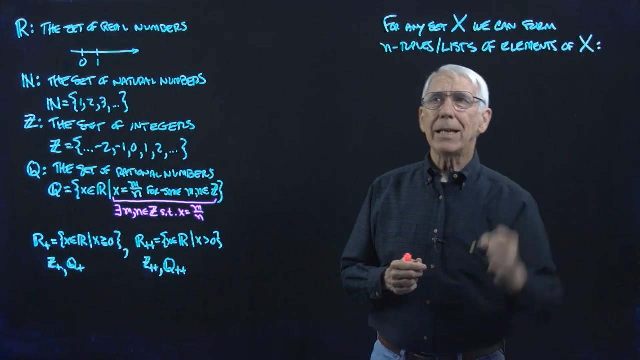 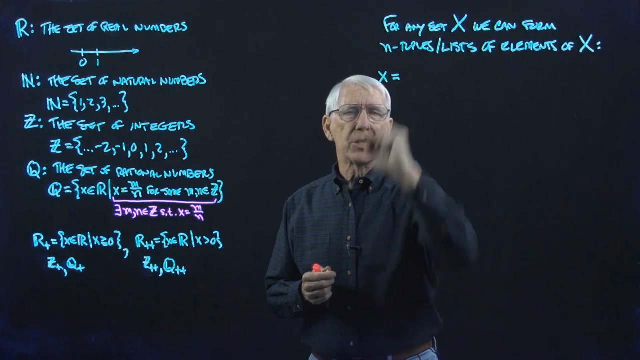 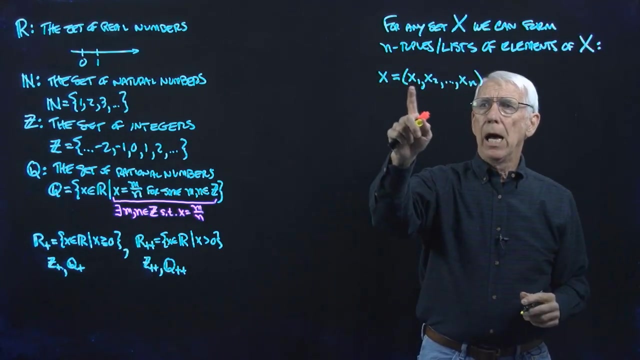 we can form what are called entuples, and we often use the word lists instead. Entuples are lists of elements or members of X, And so a typical entuple I like to call it- would use just a letter x, let's say as the name of the whole entuple or the whole list, and it would consist of a list with parentheses around it, a list of elements of x. 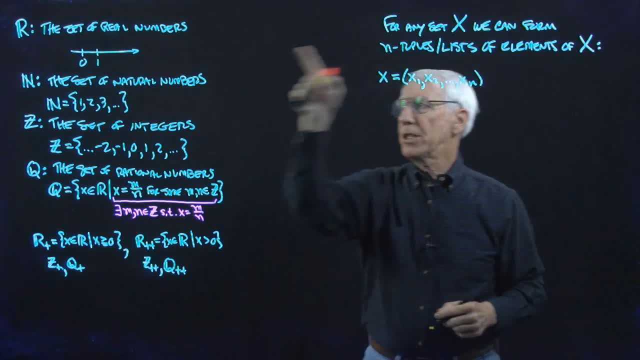 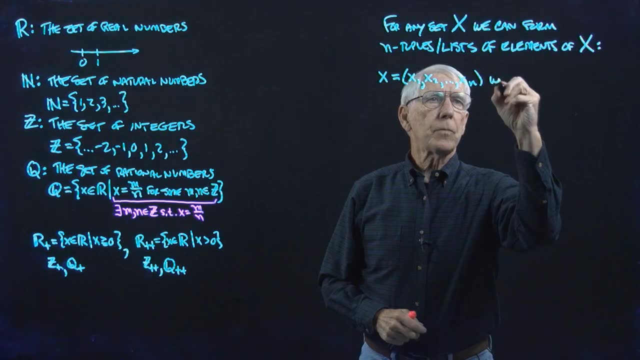 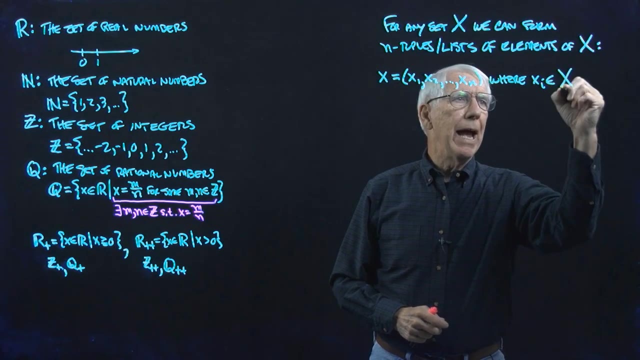 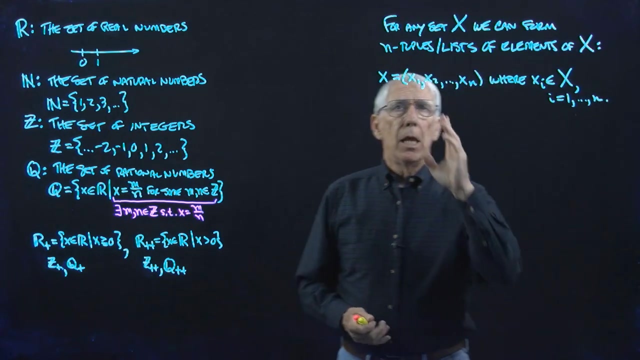 So, for example, if this is, if capital X is the real numbers, then this would just be a list of n real numbers. So where xi is in capital X and here, here we'll just write: i equals 1 to n. this would be the name of the entuple or the list. 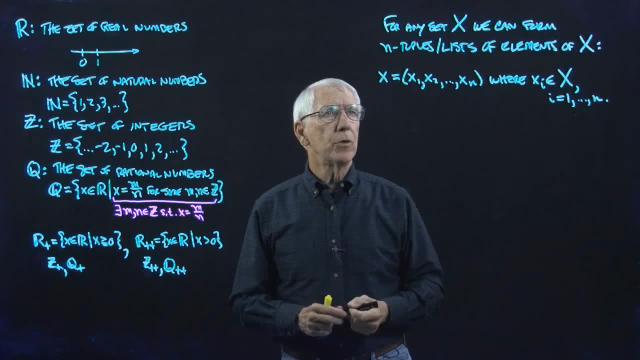 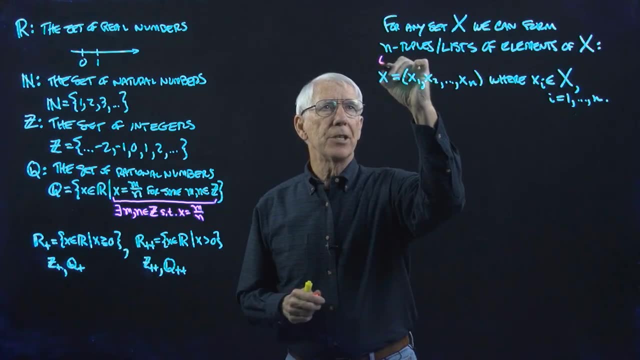 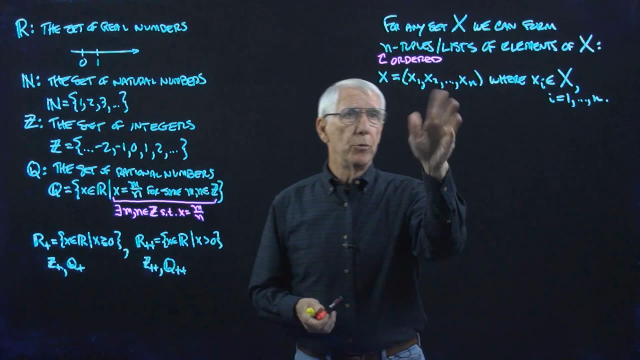 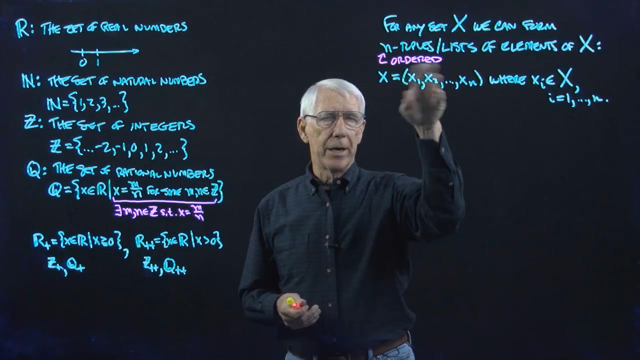 And I should point out that we often refer to these. we often add on the adjective ordered entuples or ordered lists. So let's put that down here, and the reason for that is because the order really matters here and I'm not going to say more about that right now because in just a few minutes we're going to do a couple of examples where we'll see that and I'll bring that out in a little more detail. 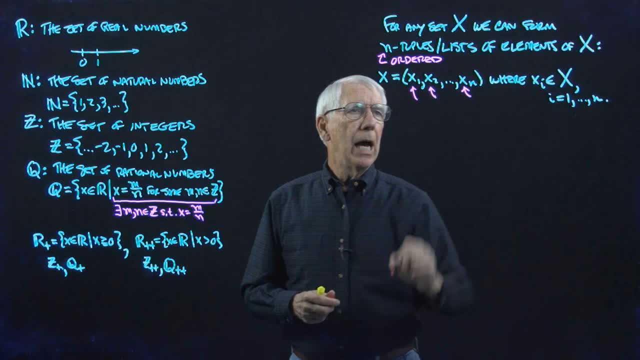 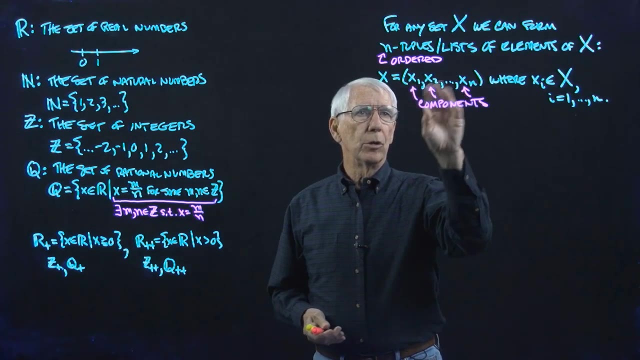 The various components of the entuples are called components, So that's the word we use to refer to the individual elements. I don't want to use elements that can be a little confusing, but the individual items in the list. Okay, and so these are the components of